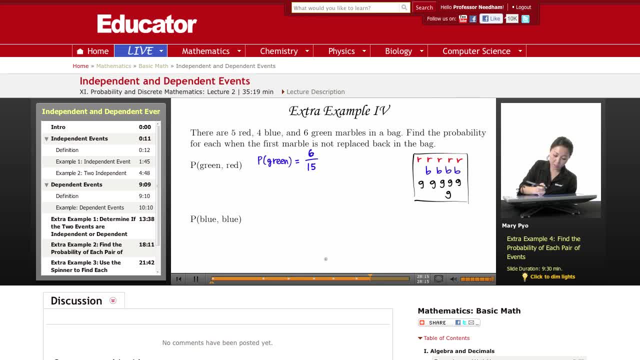 i still have to simplify it right. what number goes into both six and fifteen? they share a factor of three, so this is going to be two over five. the probability of picking a green is two over five. well then, now i have to pick my second marble, and that's going to be red. now, because that first. 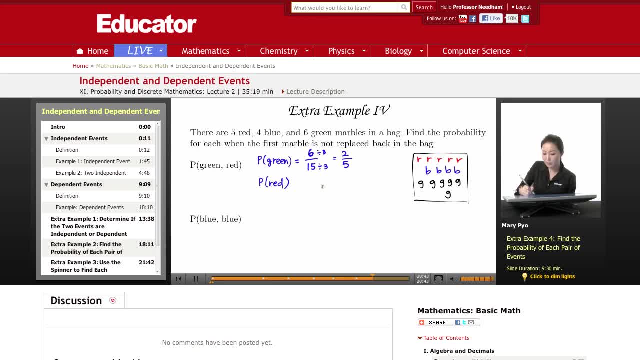 marble, the bag. this marble- one of the green- is now gone. right, it's no longer in there. so probability of picking the red. how many reds do i have? i have five red marbles, five on top over. how many marbles do i have now? well, after that one's gone, i have 14 left right. 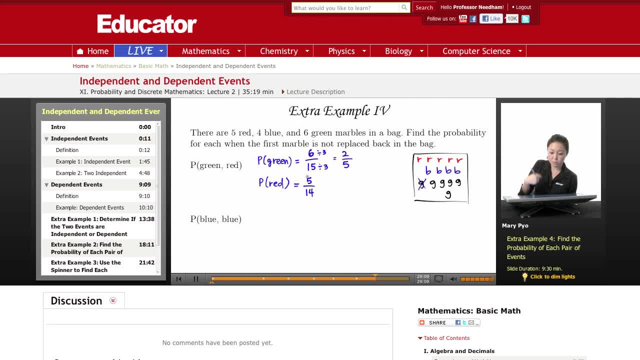 so it was 15, and then minus the one that we already picked, so that's 5 over 14.. okay, so the probability, and now this fraction. i can't simplify right. so that's the probability of picking the red. so now i can. to find the probability of both happening, i take this one. 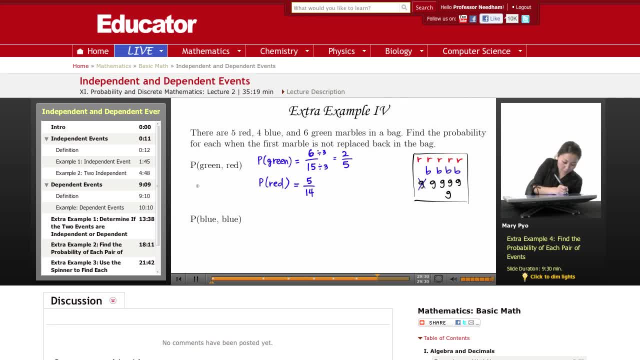 and i take this one and i multiply it together, so it'll be probability of the green times, the probability of picking the red, and this is dependent, so it's the red after green. so 2 over 5 times 5 over 14.. 2 times 5 is 10, 5 times 14, 14 times 5. you do this right. that's 20, 5 times 1. plus the 2 is 70. 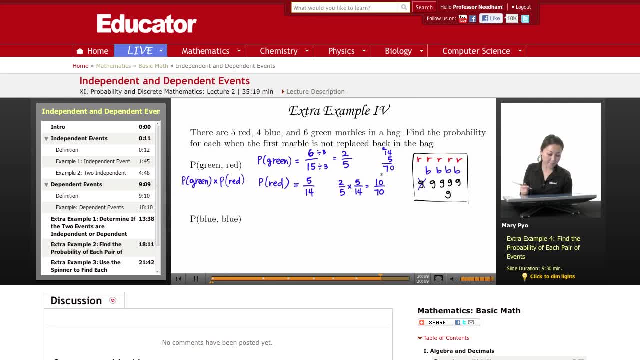 2 times 5 is 10. 5 times 1 plus the 2 is 70, now fraction. so i have to simplify it. what number goes into both top and bottom 10? so i divide by 10 for each, i get 1 over 7 as my answer. so the probability of picking a green. 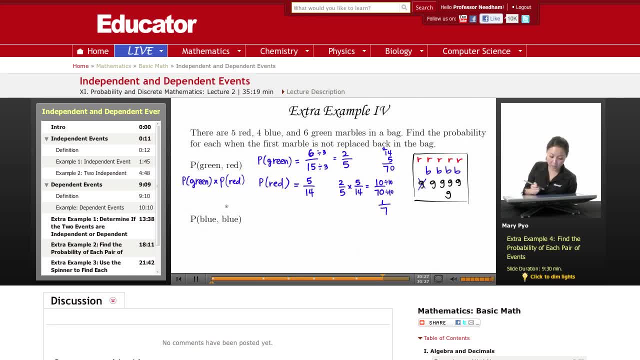 and then afterwards, without replacing it back in, picking a red marble is 1 over 7.. okay, let me write this for this second problem. now we want to find the probability of picking a blue and then afterwards, without replacing it back in, pick another blue. so again, two dependent events. so probability picking the first blue, the first. 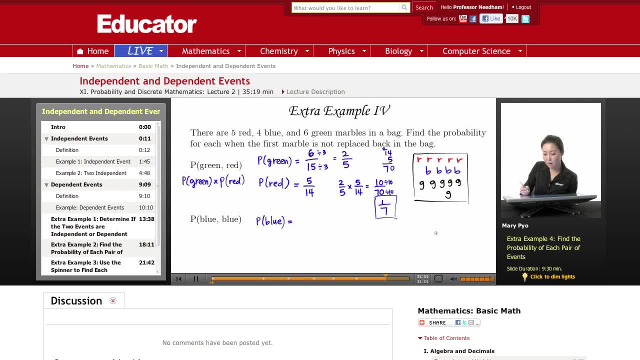 event. what's my desired outcome? how many number um, or how many blue marbles do i have? here in the back i have four blue over a total of 15 marbles. so the probability of picking up blue marble is 4 over 15. i can't simplify it, so that's the probability. and then for my second pick, 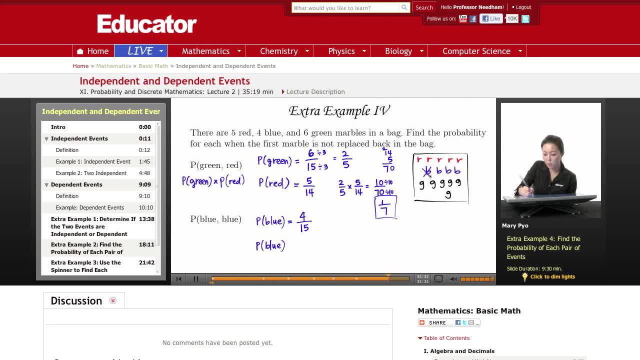 because, again, it's not being replaced in the bag. this one is no longer in the bag, so i have one less marble. So for my second pick, I want to look at how many blue marbles I have left. I have three left, I had four, but one's gone. 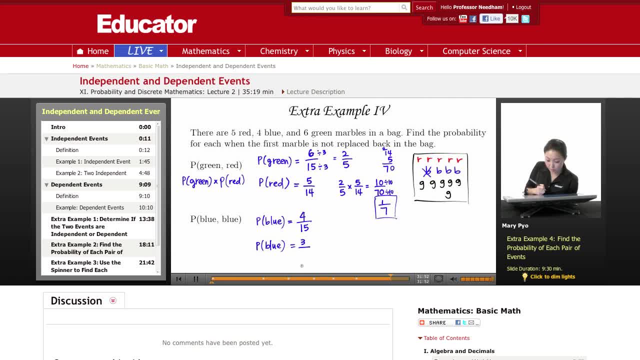 So now I have three over And then I don't have 15 anymore. I have 14 now. So probability of picking the first blue was 4 out of 15, because I had all my blue, which is four of them out of a total of 15 marbles. 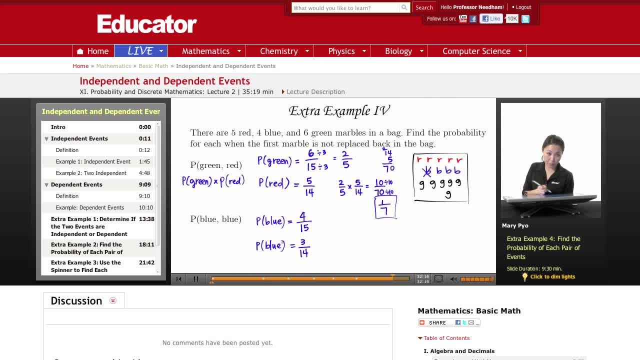 For my second pick. I'm also wanting to pick another blue one. I only have three left because the first one was replaced back in, out of a total of 14 marbles left. So now I'm going to take the first event and then multiply it to the probability of the second event happening. 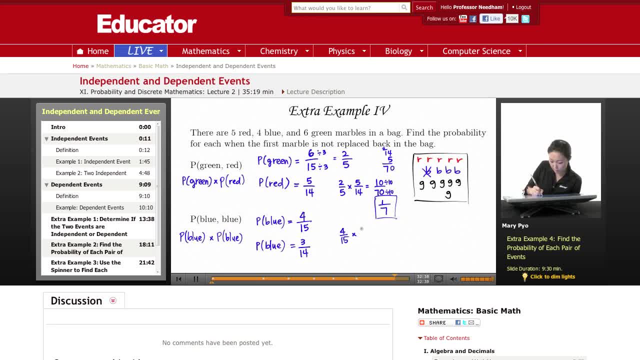 So it's 4 over 15 times 3 over 14.. 4 times 3 is 12 over 15 times 14.. Okay, I'm going to multiply it. This is 20.. 4 times 1 is 4, plus 2 is 6.. 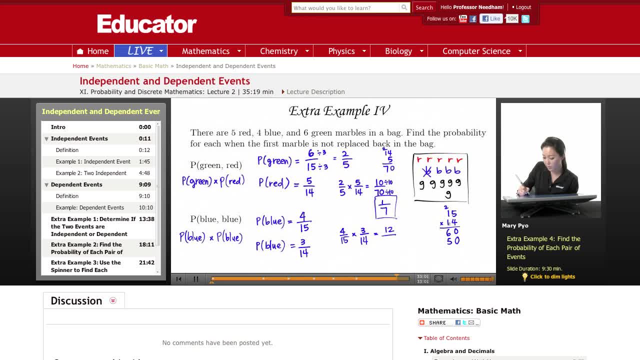 Okay, I'll leave the space alone. 1 times 5 is 5.. 1 times 1 is 1.. I'm going to add them down: 0, this is 11, this is 2.. So 210.. 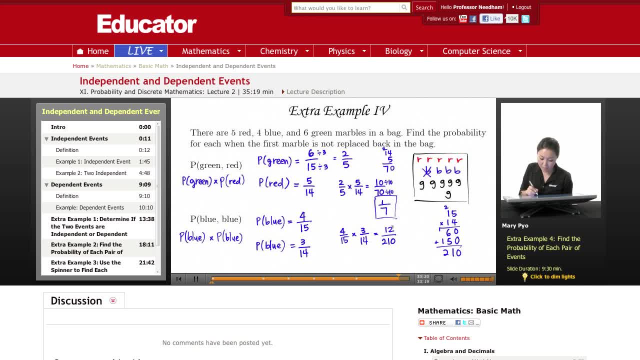 Okay, now I know I can simplify this fraction, because this number is an even number and this number is an even number, So let's divide each of these by 2.. Oops, So 12 divided by 2 is 6 over this. 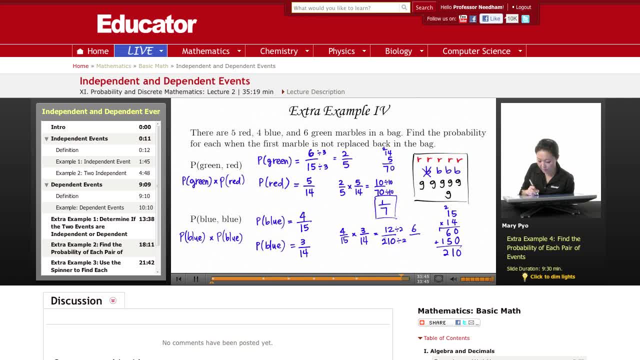 If I take the 200 and I divide it by 2, I get 100.. So this divided by 2 is 100. This divided by 2 is 5.. So if I divide the whole thing it'll be 105.. 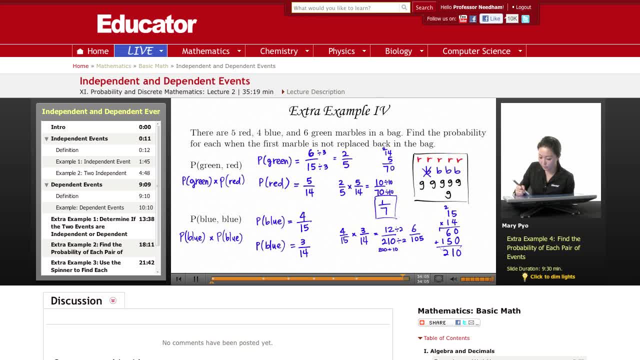 Okay, Now it looks like 6 over 105.. I also have another factor, So I can divide this again by. I know 3 goes into that one and 3 also goes into this one. So 6 divided by 3 is: 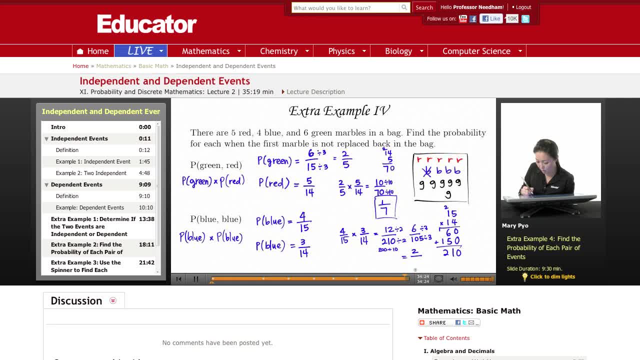 write it down here: 2 over 105 divided by 3. Okay, let me show you that one. So 3 goes into 10 three times. That gives you a 9.. Subtract it, I get one left over. 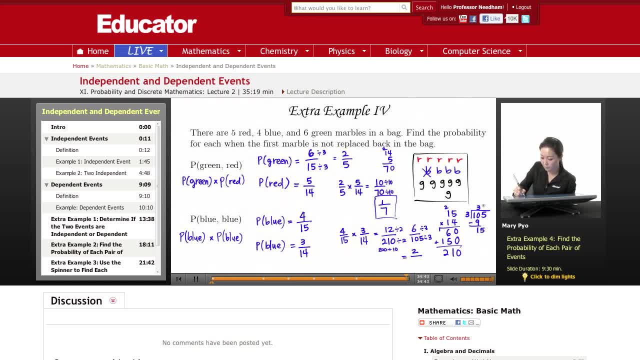 Bring down the 5.. 3 goes into 15. five times, That gives you 15.. We subtract it. I have no remainders, So my answer is 35.. Okay, can I simplify this further? Okay, no, I can't, because this is not an even number. 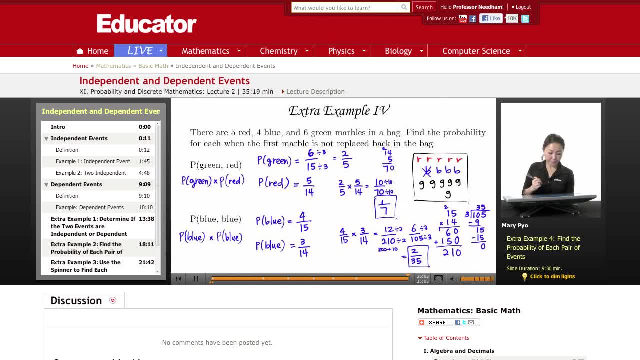 So this is my answer. So again, finding the probability of of two events, you have to find the probability of each event occurring and then you're going to multiply them together, whether it's independent or dependent events. And that's it for this lesson.